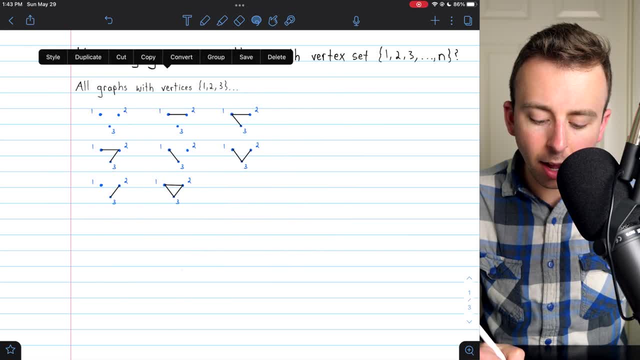 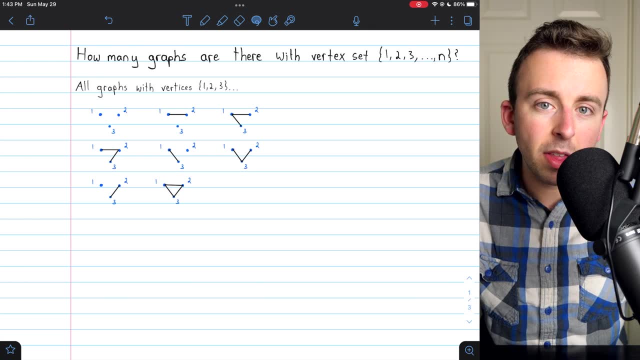 this video, Graphs that have the same structure- you may or may not know- are called isomorphic graphs. So we're counting all graphs on N vertices, even if some of them happen to be isomorphic. Now, enough of that, Let's go ahead. 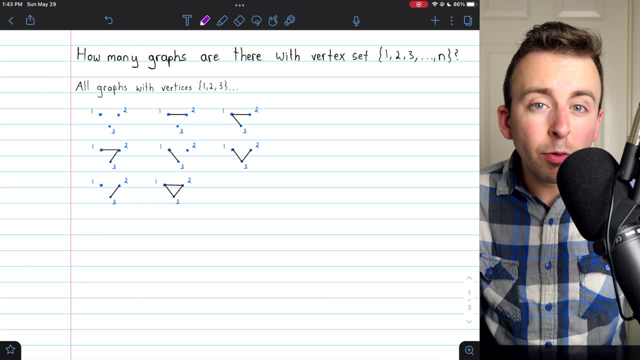 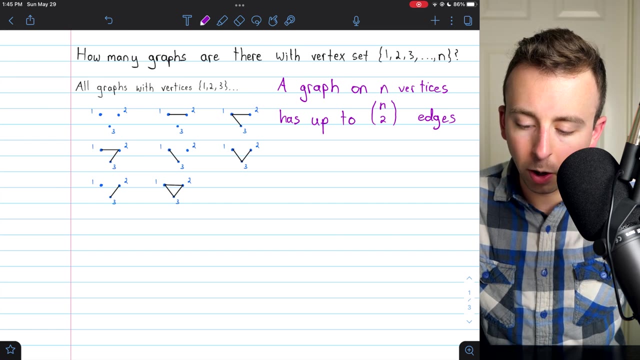 and actually answer the question. It doesn't take too long. The first thing we need to address is how many edges could a graph on N vertices possibly have? The answer to that question is pretty simple. It's just N. choose 2, a binomial coefficient or combinations. 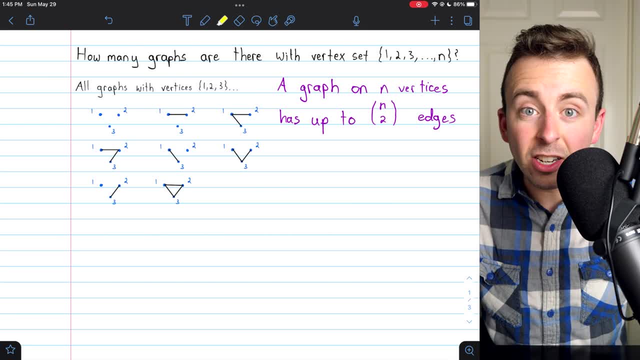 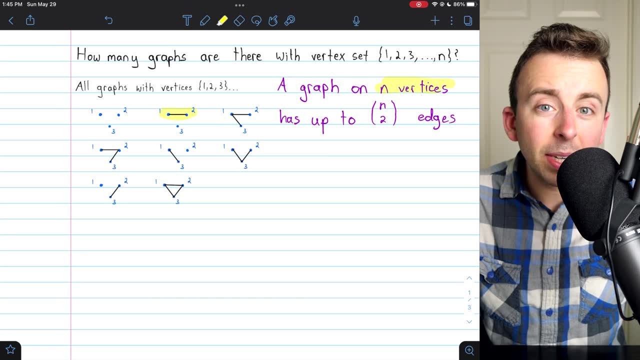 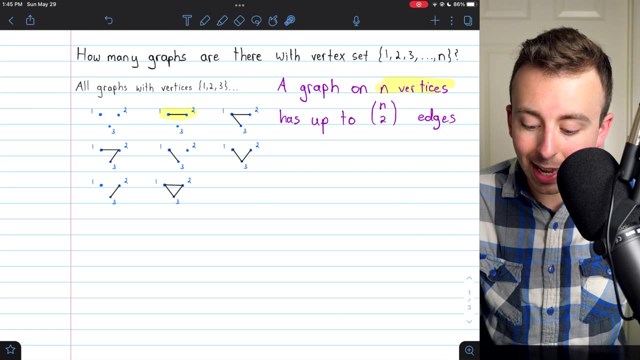 if you think of it that way, This is because each edge joins exactly 2 vertices. So if our graph has N vertices, how many edges could it possibly have? How many possible edges are there? Well, it's just the number of ways that we can pick 2 vertices from a collection. 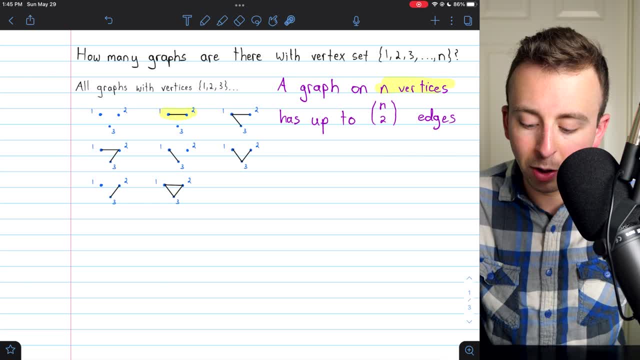 of N vertices, which is the binomial coefficient, N choose 2.. For example, on a graph with 5 vertices, there are 5 choose 2 possible edges and this is equal to 10.. So there are 10 possible edges on 5 vertices. So we can pick 2 vertices from a collection of N vertices. So we can pick: 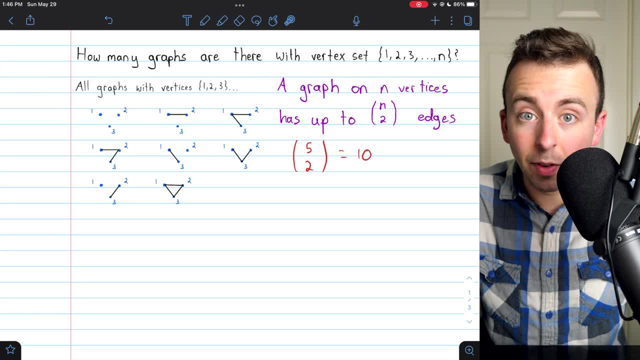 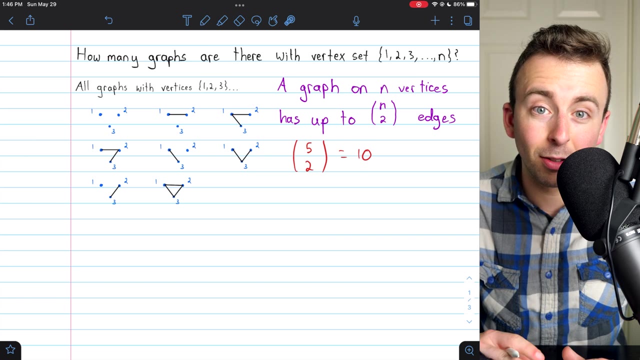 5 vertices, because any 2 vertices give us an edge. So we just need to count how many ways can we pick 2 vertices from our collection of 5.. This, of course, also means that on a complete graph with 5 vertices there are 10 edges, because those are all the possible edges. All right, so we know. 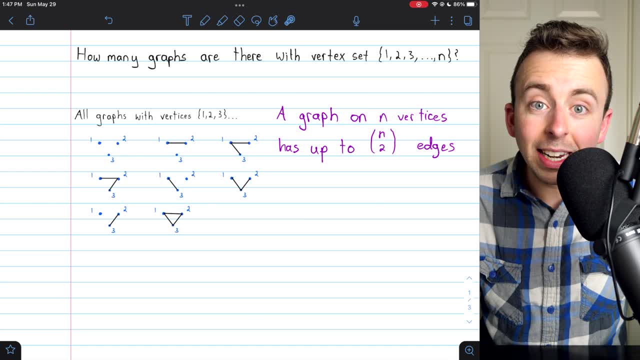 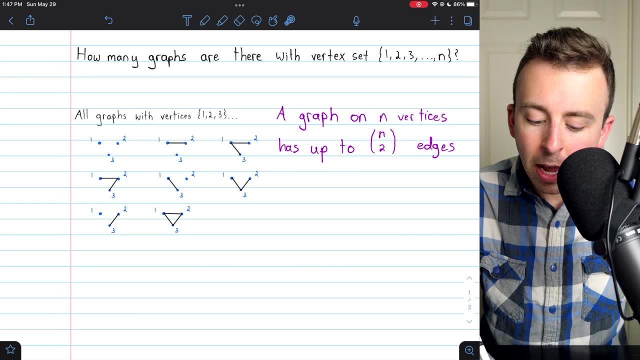 our graph has vertices 1 through N. We know that it could have up to N choose 2 edges. So how do we pick 2 vertices from a collection of N vertices? Well, for each of the N, choose 2 edges. there are. 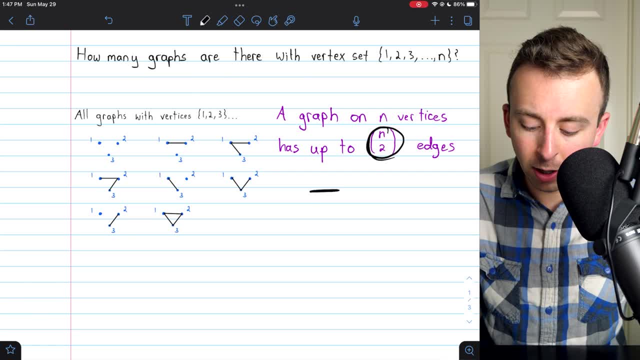 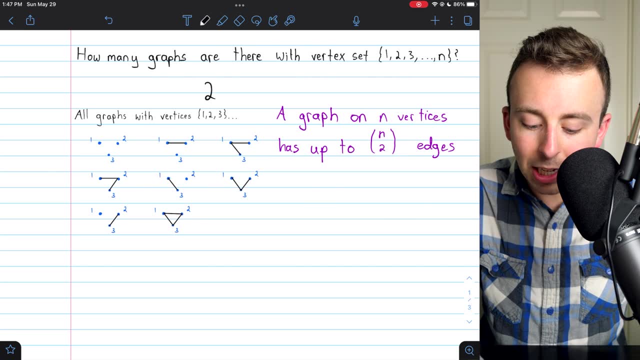 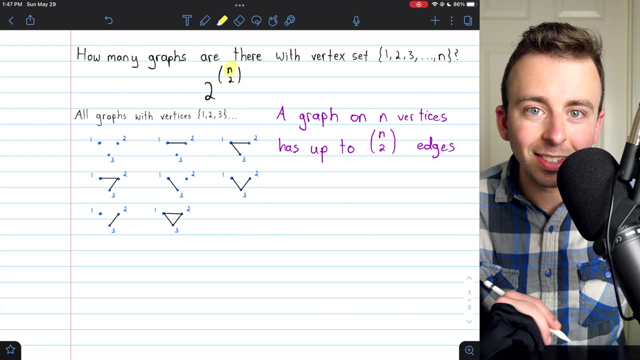 2 possibilities. Our graph could have the edge or it could not have the edge, And so the answer is quite simple: It's just 2 to the power of N, choose 2.. That's the number of graphs on N vertices. 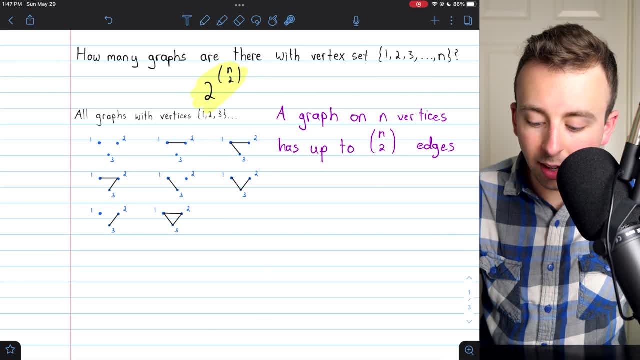 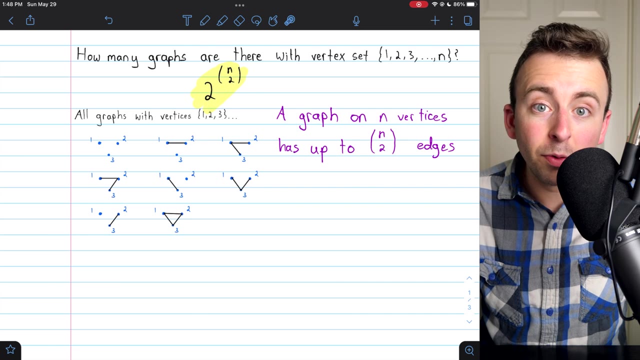 Again. that's because the number of vertices is fixed. We're saying we've got N of them labeled, 1 through N. Then all that remains to be decided are the edges, And there are N. choose 2 possible edges and there are 2 options for each one. You can have it or you cannot have it. This is very much. 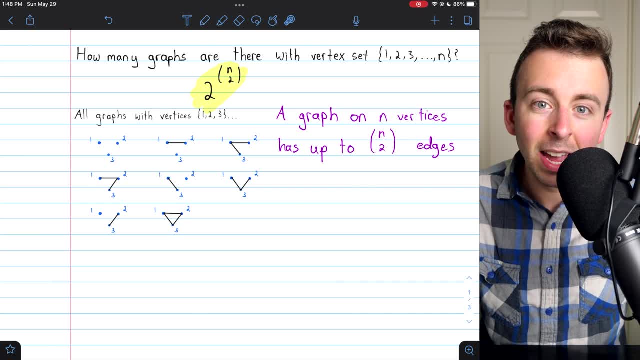 like counting subsets, if that's something you've done. So we just have to raise 2 to the power of the number of possible edges. That gives us the number of possible graphs, where, of course, we are counting labeled graphs, So we may be counting isomorphic graphs multiple times. 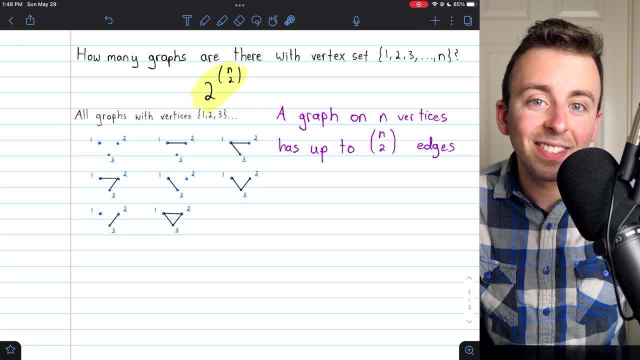 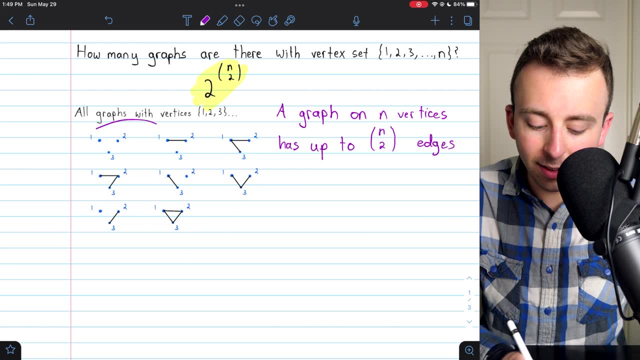 because they are different, even though they have the same structure. Try out this formula for yourself. I'll go ahead and write it out for the 3 vertices situation, since I've already gone through the trouble of drawing out all of those graphs. So the formula tells us for 3 vertices. 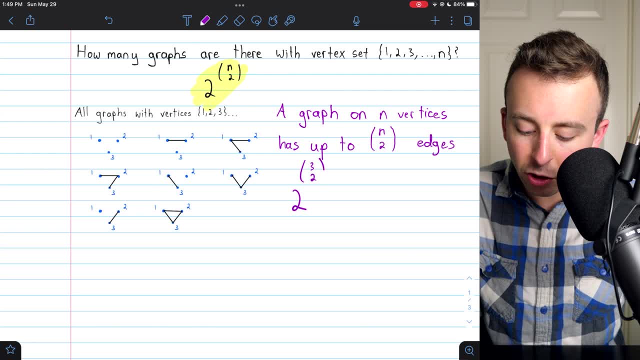 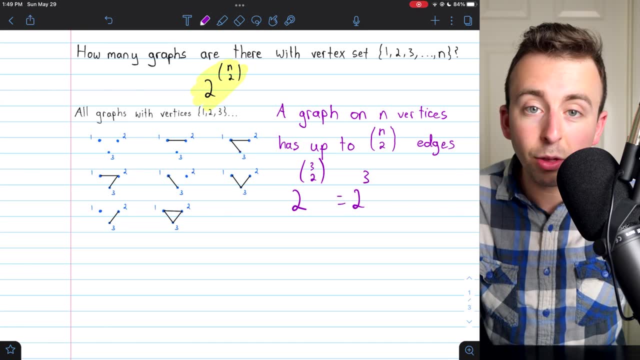 there should be 2 to the power of 3. choose 2 different graphs. 3 choose 2 is 3, so this means there should be 2 to the 3 different graphs And, of course, there should be 2 to the power of 3. choose 2 different graphs. 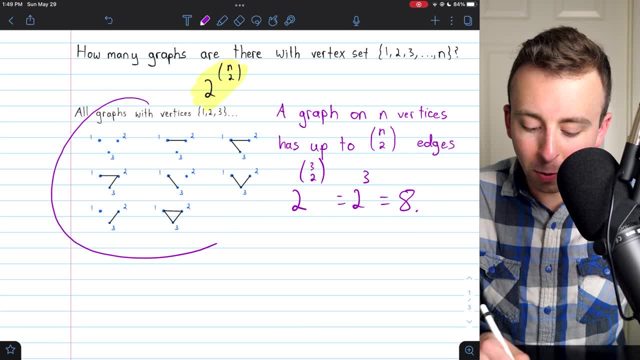 2 plus 1, huh, Or what do you mean? 0 nya re, 0 nya' 80 odd, OK, old opted. course that's eight, which agrees with this list here, And that's really it. But as far as counting, 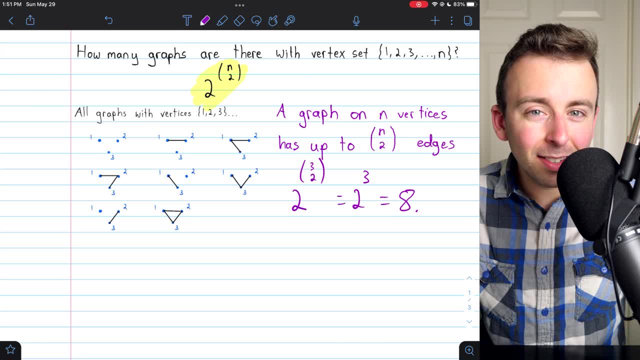 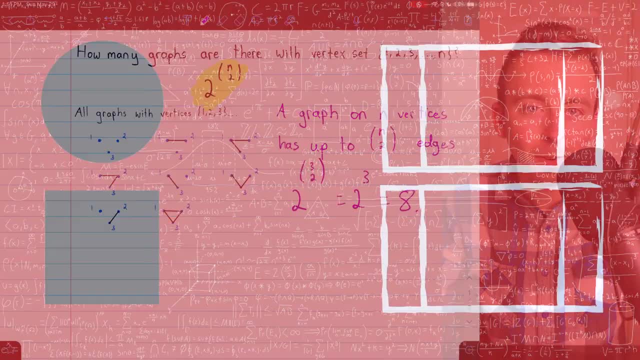 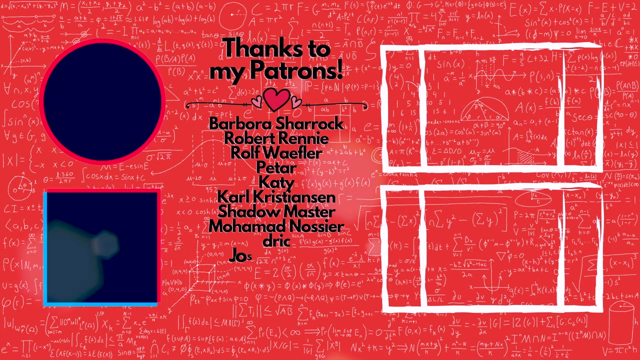 non-isomorphic graphs goes. that's considerably more complicated, but it can be done, So we'll save that for another time. I'll leave a link in the description. I could be happy.